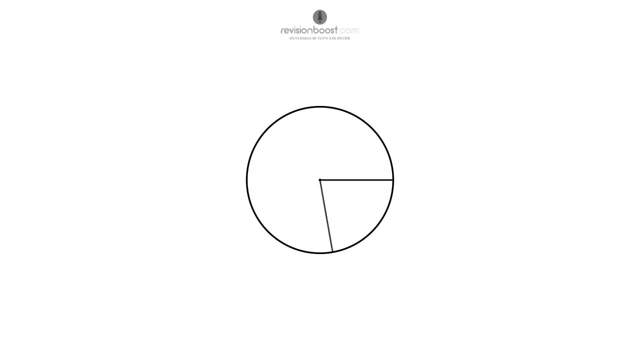 to draw one radius here and another radius there, like that. By the way, the plural of radius is radii, so we would say that we have drawn two radii on this circle here. What I'm going to do is I'm going to connect the two points where these radii touch the circumference of the circle. 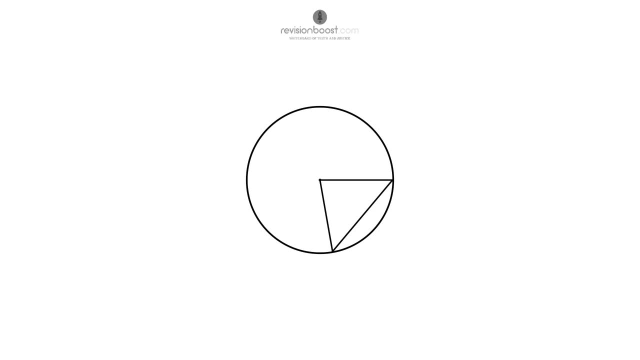 with a line just like this. You can see here that we've formed a triangle. now we know from our definition of the circle that these two lines, the radii, are going to be the same length. Now this means that the angles opposite those lines are also going to be the same. 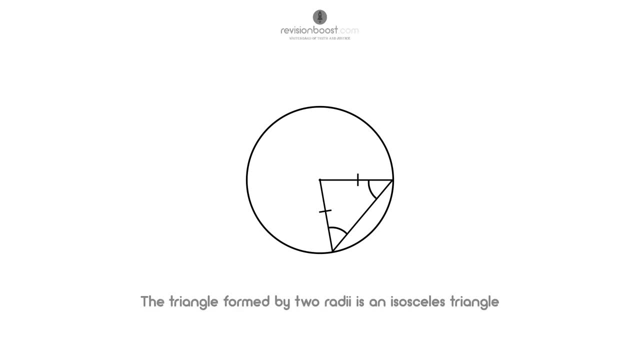 size. As a result, we can say that the triangle formed by two radii in a circle like this is always an isosceles triangle, And that is rule number two. If you were to pick any two random points on the edge of a circle and form a triangle using those two points, with the 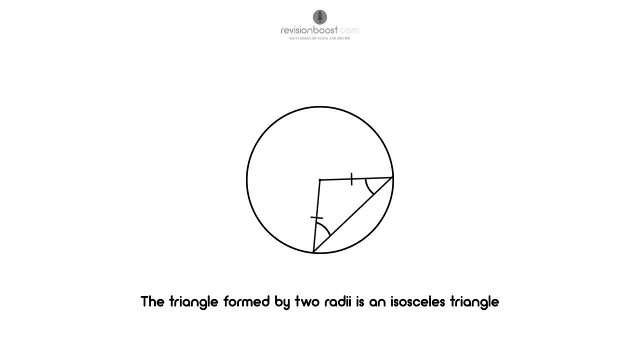 center, then the triangle that you form is always an isosceles triangle. To understand rule number three, we first need to take a look at what a chord is. Now remember when we're drawing straight lines on the same diagram as a circle. there are three possible scenarios. 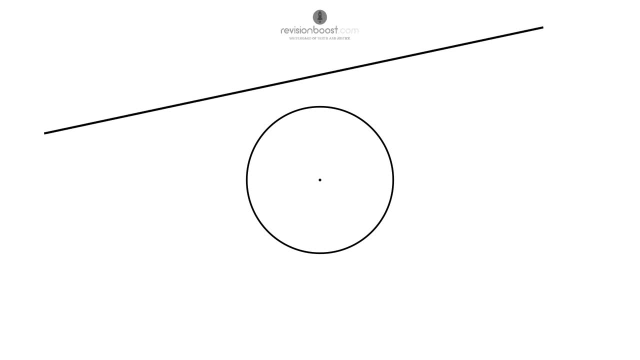 Either the line misses the circle totally, or the line just touches the edge of the circle once and is a tangent, or the line passes through the circle twice. Now there are two types of line passes through a circle twice. If the line passes through the circle twice and goes through the 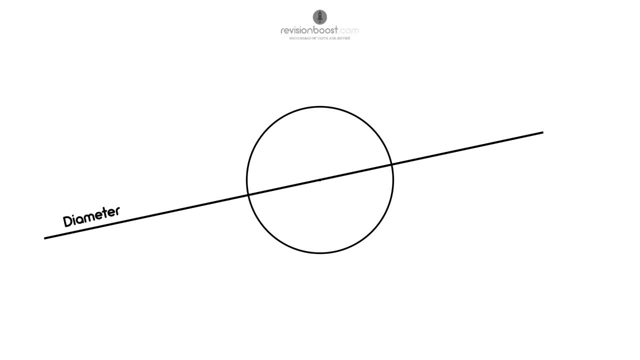 center. we call it a diameter. If a line passes through the circle twice and doesn't go through the center, this is called a chord. So you can see: all of these lines on here are chords of the circle. Now, rule number three says that the perpendicular bisector of any chord always 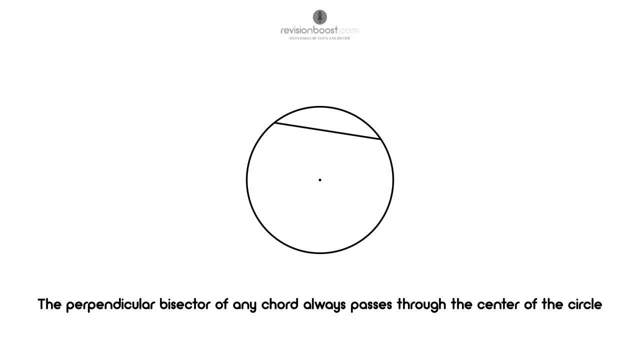 passes through the center of the circle. At this point you're probably wondering what on earth is a perpendicular bisector? Well, there's two parts to this: perpendicular and bisector. First of all, a bisector is just a line that passes through the center of another line. So from this we can see: 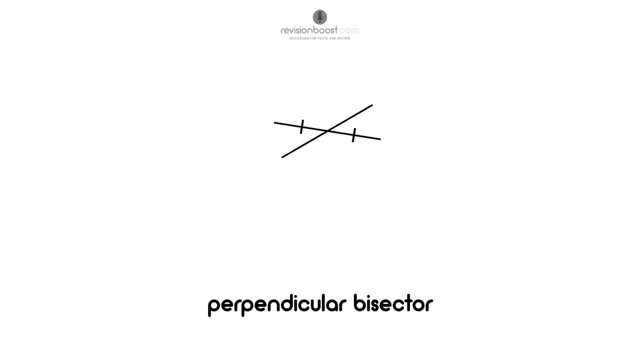 that a perpendicular bisector is a line that passes through the center of another line at a right angle. So overall rule number three says that if you draw any chord on a circle like this and then draw the perpendicular bisector of that chord, this will always pass through the center of the circle. 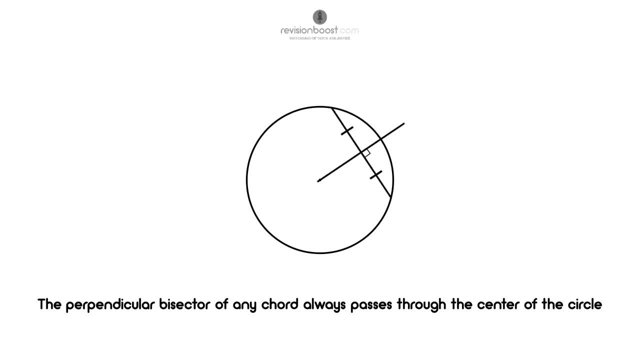 Now, to prove that I'm not lying to you and that this is definitely correct, I've put another fancy animation on the screen here You can see. no matter what chord we draw, the perpendicular bisector always passes through the center of the circle. Rule number four says that if we draw any 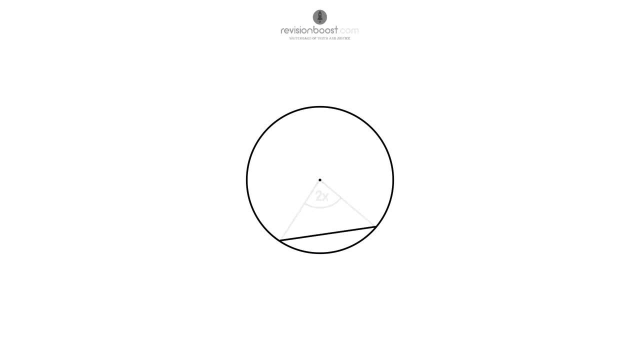 chord on the circle, the angle formed at the center is always double the angle formed at the circumference, As you can see here. here, it doesn't matter how we draw this diagram: for any chord, the angle at the center of the circle is always double the angle at the edge of the circle. Now, 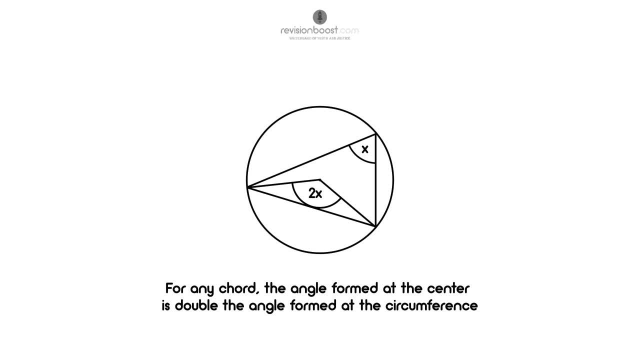 a lot of the time, GCSE examiners will try and catch you out by not including the chord on the diagram that they draw, So what I'd recommend doing is looking out for this arrowhead shape. Looks kind of like a computer mouse Anytime you see. 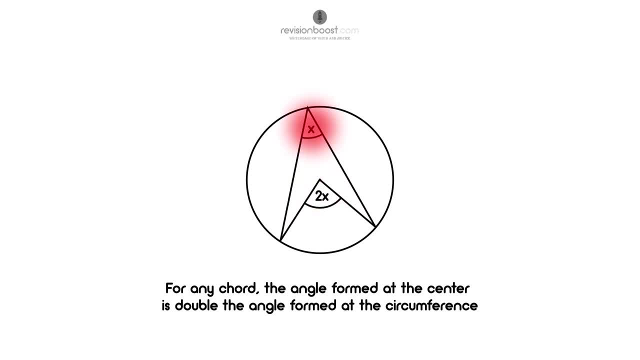 the shape. the angle here is always double the angle here. Now, if the examiners are being really sneaky and they're really determined to catch you out, they'll first of all draw the diagram without the chord, but then they'll also draw the diagram like this, so you can't recognize the arrowhead. 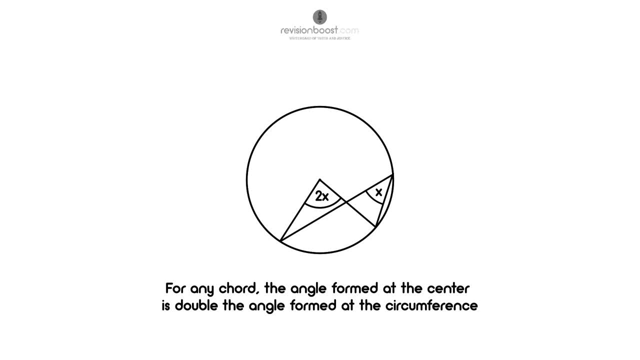 shape. So this is just another thing to look out, for You can see, even when we draw the diagram like this, the angle at the edge of the circle is always half the angle at the center of the circle. Nice Rule number five is a special case. 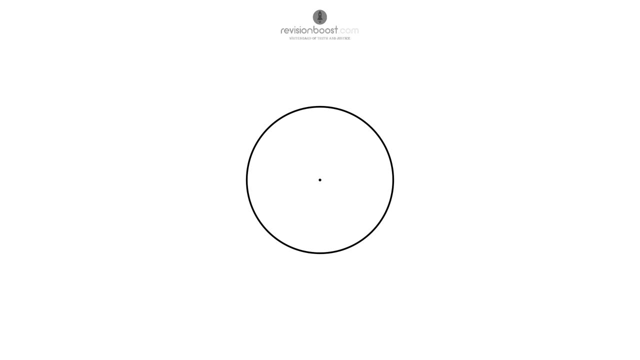 of rule number four. Now, remember: rule number four says that if we have any chord, the angle at the edge of the circle is always half the angle at the center. Now, this means that if we were to draw a diameter just like this, you can see how the angle here at the center is 180 degrees. 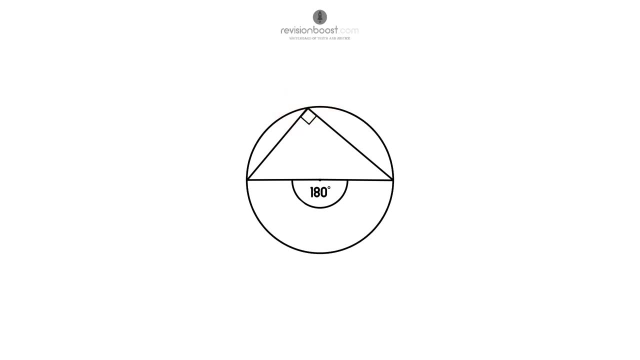 Now, this means that the angle at the edge of the circle will be 90 degrees. So rule number five says that if you have a semicircle like this, the angle in that semicircle is 90 degrees. Rule number six is basically the same as rule number four as well. 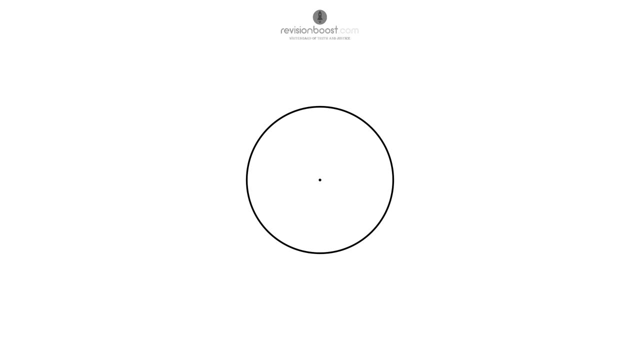 But before we get into rule number six, we first need to understand what a segment is. Whenever you draw a chord on a circle, the two shapes either side of that chord are called segments. Now rule number six says that whenever you draw a chord, the angle in each segment is: 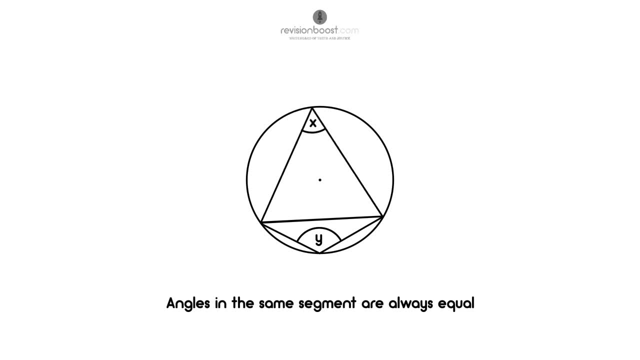 always the same. So you can see how this angle, no matter what we do, is always the same, and this angle here is also always the same. As you can see, this is very similar To rule number four. Rule number seven says that opposite angles in a cyclic quadrilateral always add up to 180 degrees. 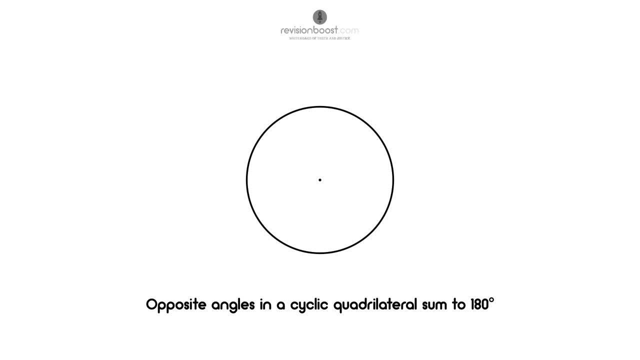 Now, from this, you're probably wondering what on earth is a cyclic quadrilateral? Well, if you were to draw a circle and then put four random points on the circumference of that circle and connect them together, drawing lines like this, what you have drawn is a. 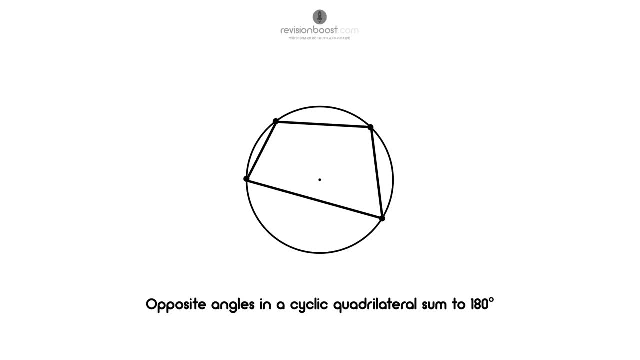 cyclic quadrilateral. So really a cyclic quadrilateral is just a quadrilateral where all of the vertices of the quadrilateral lie on the circumference of a circle. Whenever you see one of these cyclic quadrilaterals on an exam question, because of rule number seven, you know that the opposite angles in that cyclic quadrilateral 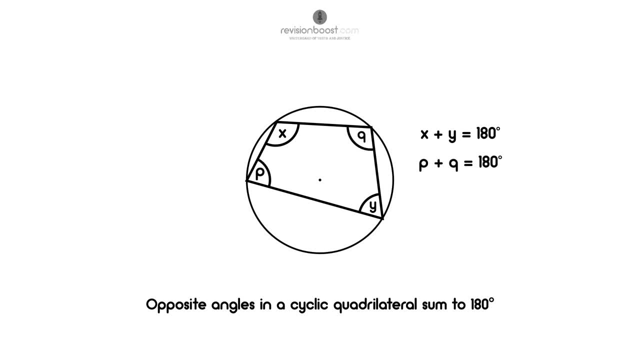 always add up to 180 degrees. Now it's really common for examiners to try and catch you out using this rule as well. The way they do this is by drawing a shape that looks like this: Now, the common mistake that students make is that they think rule number seven applies to this. 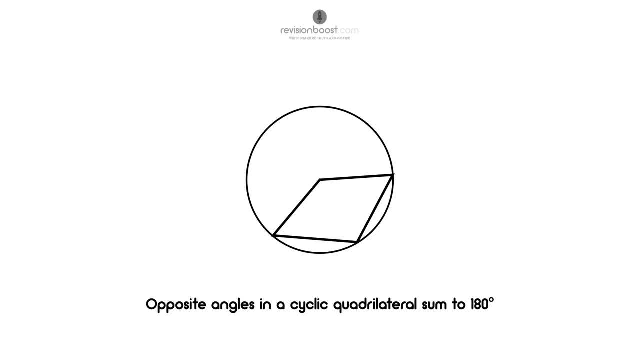 diagram and that the opposite angles in this shape add up to give 180.. But this is not true at all. The reason it's not true is because this shape here is not a cyclic quadrilateral. This point here is at the centre of the circle, not on the circumference. 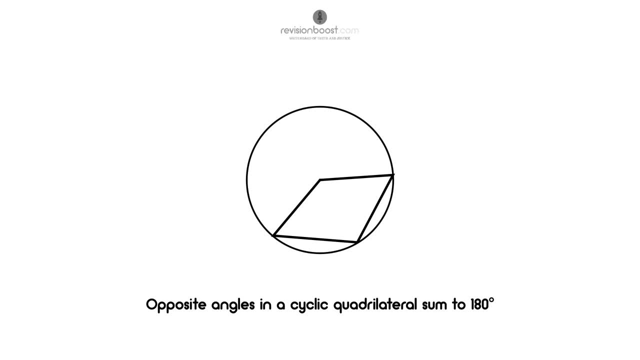 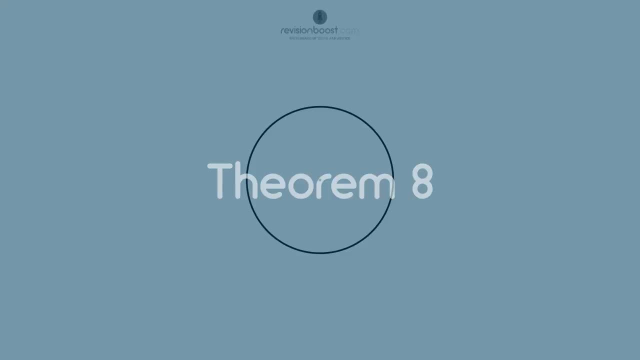 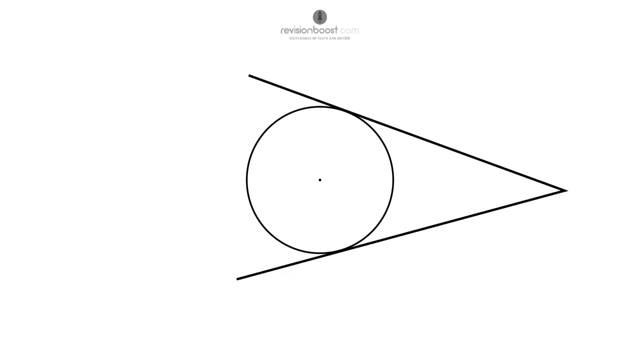 So before you apply rule number seven, just make sure that all four of the points lie on the circumference of the circle and not anywhere else. Alright, nearly there, only two rules left. Rule number eight says that if we were to draw two tangents on a circle, the distance between 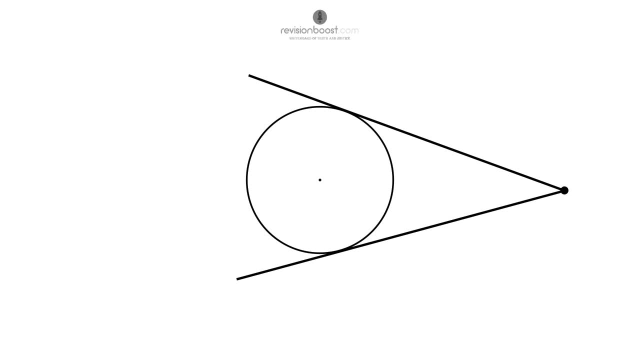 the points where those tangents cross each other and the points where the tangents touch the circle is always equal. So you can see, no matter how we draw this diagram, these two lines here are always equal in length. Now, because we know that these radii are also 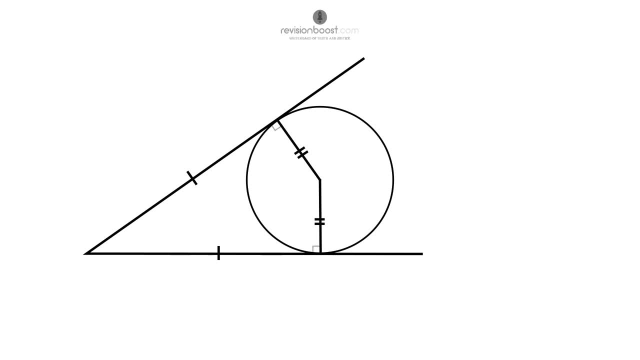 equal in length, and we also know that the angle between each of these tangents and the radii is always 90 degrees. this means that if we were to draw a third line like this, forming two different triangles, these triangles are both exactly the same. They have the same size.